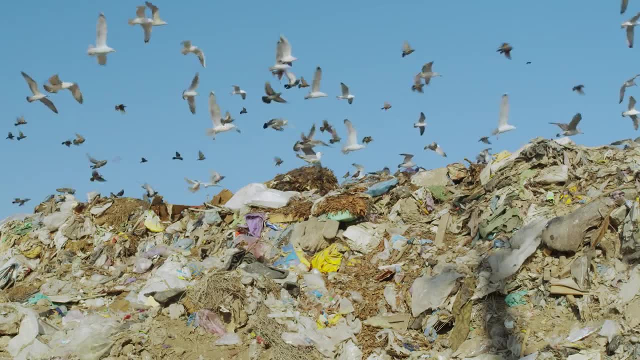 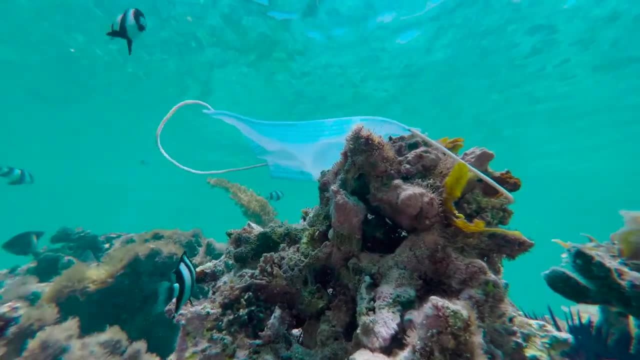 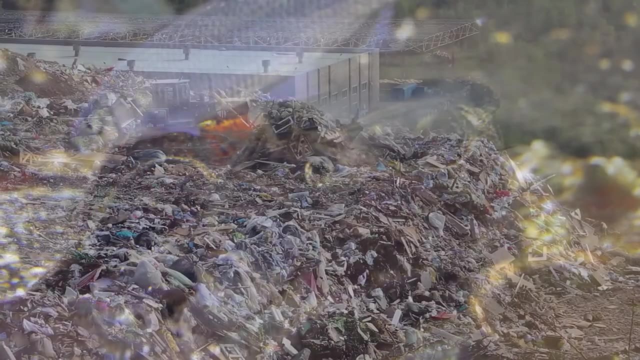 That's producing plenty of issues, such as coastal flooding and human-made climate change, And what's worse is that there are now so many bits of junk floating around in our oceans, affecting aquatic life negatively. Human garbage has long been harmful to our environment. 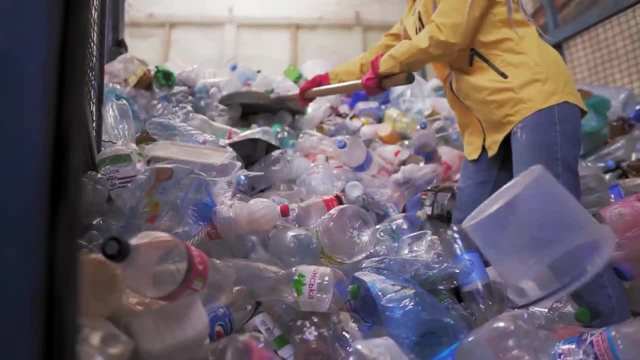 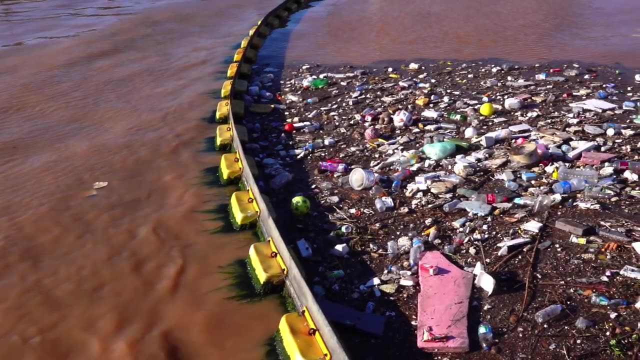 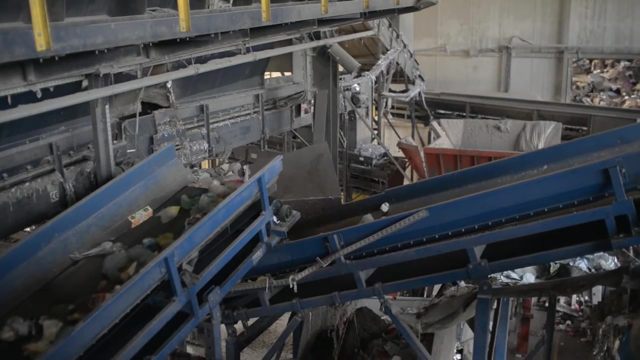 Humans produce far too much waste and are incapable of dealing with it in a sustainable manner. Non-biodegradable waste that can't be recycled correctly is polluting our oceans and landfills. According to a recent study, just 9% of the 6.3 billion metric tons of plastic trash 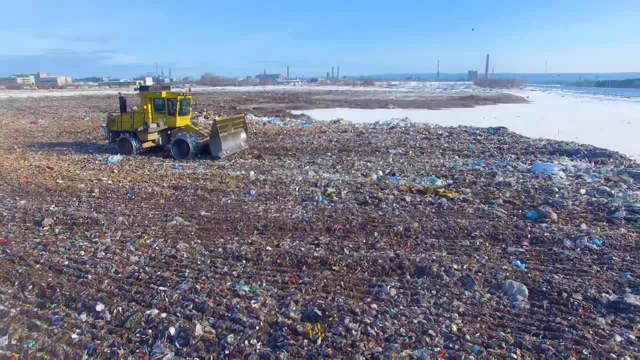 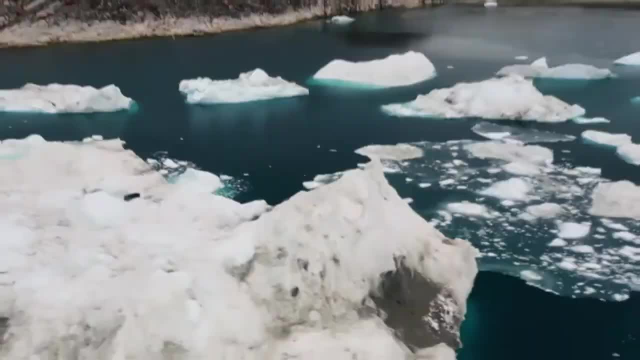 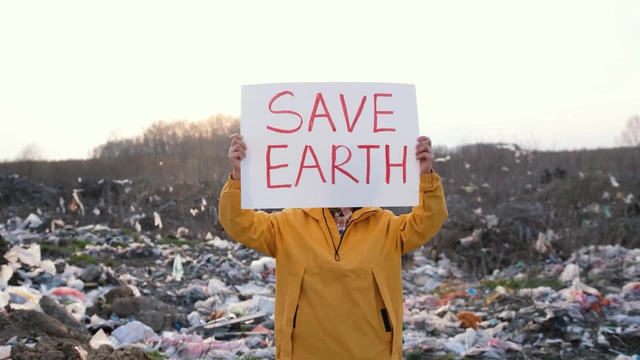 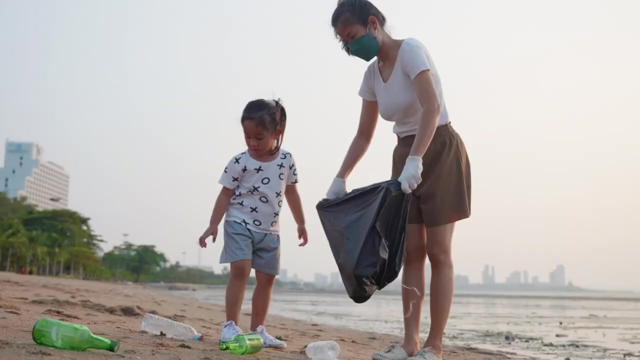 have been recycled. Overall, the amount of garbage generated has a detrimental influence on the environment in several ways. These include its contribution to the worsening climate catastrophe, its poor impact on wild life, the natural environment and its harm to our public health. So stay tuned to find out what is the impact of our waste. 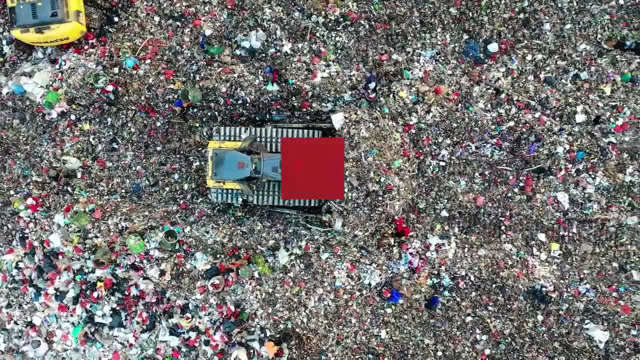 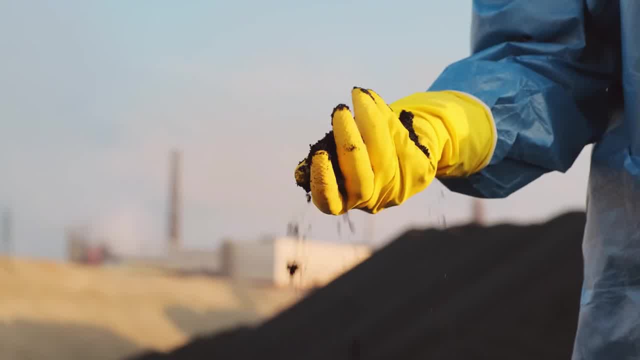 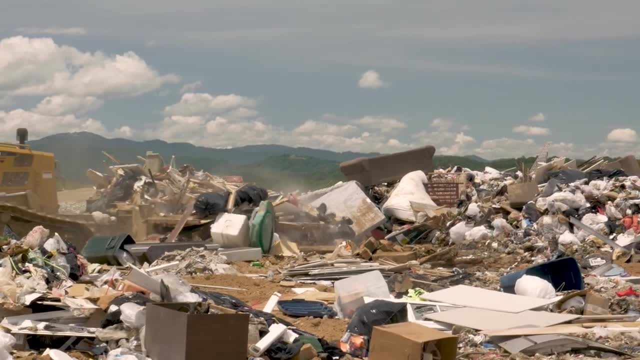 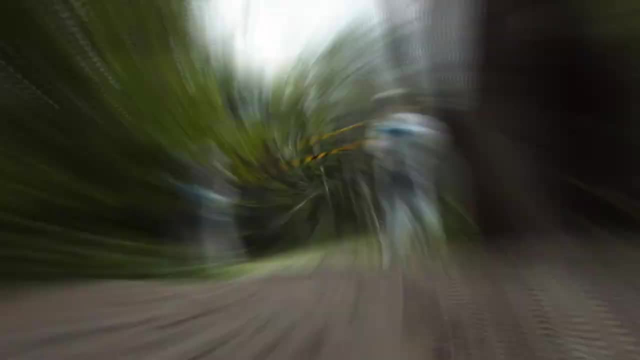 But before we begin, support this video and channel by leaving a like right now and smashing the subscribe button. Enjoy. Soil Contamination Poisons are discharged into the environment when waste is disposed of in a landfill, contaminating the soil around the dump and damaging nearby habitats. 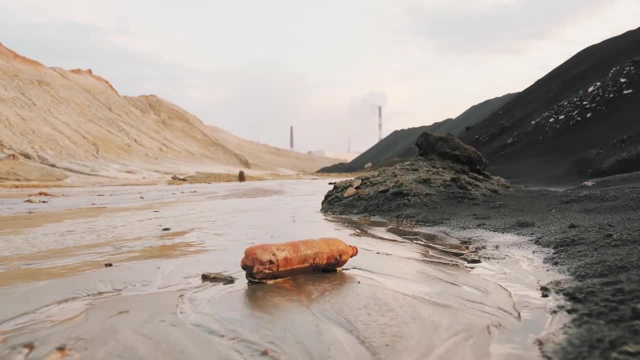 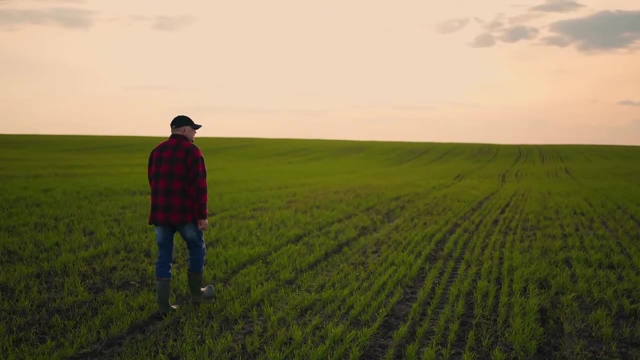 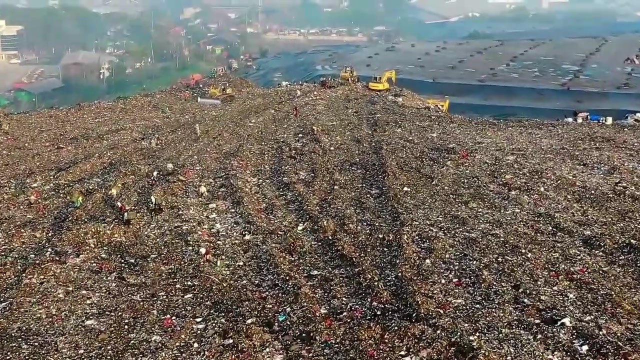 Exposure to hazardous materials and chemicals may endanger plants and animal life. The soil is an essential part of the environment and we rely on it to help grow our food. If it becomes polluted, we have to do something about it before it's too late. 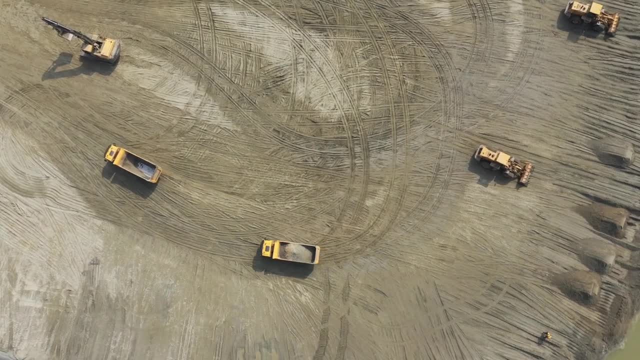 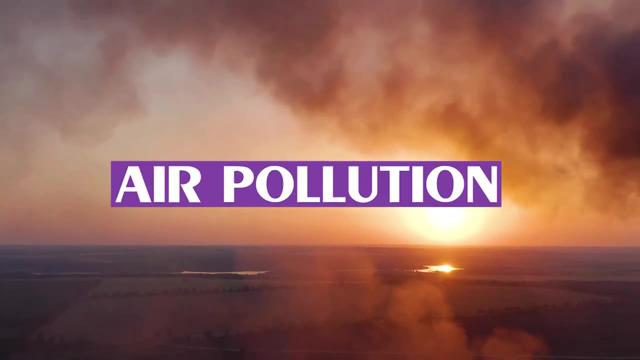 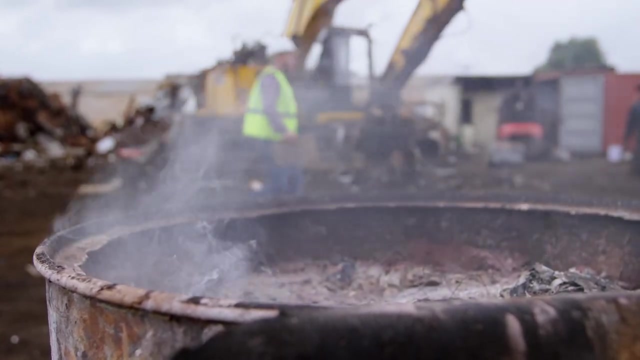 Restoring poisoned soil will cost a lot of money and effort to restore the poisoned land. Air Pollution- Another detrimental environmental impact of waste collection is the creation of air pollution. Trash frequently has a stench, indicating that it emits chemical vapors into the surrounding area. 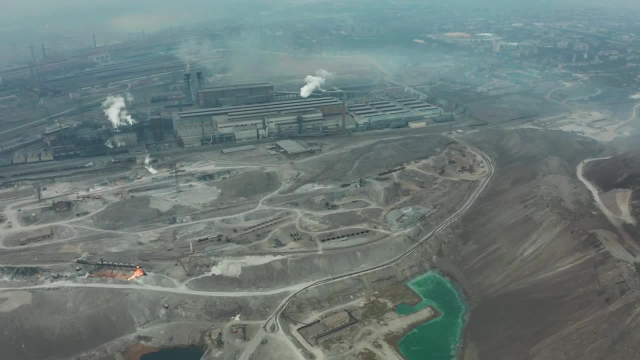 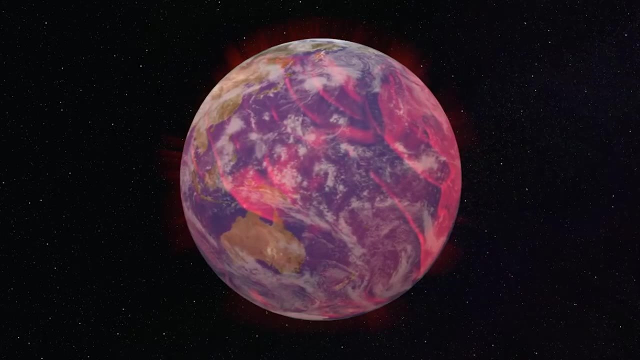 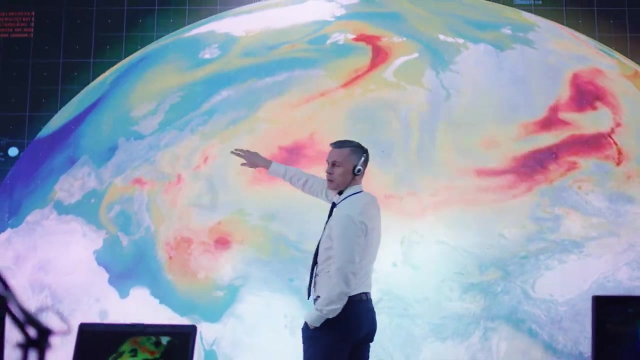 Air pollution is widespread near landfills and incinerators. These facilities also emit methane into the atmosphere, which is a major contributor to the greenhouse effect. This is raising the temperature of the Earth's atmosphere, which has the potential to be life-threatening in the long run. It also adds to acid rain, which has a variety of harmful consequences on the water cycle. It ruins numerous wildlife habitats and houses. Water Contamination, Waste collection or removals contribute to water pollution. When harmful chemicals and pollutants accumulate near waste disposal plants, they will run off into neighboring water. 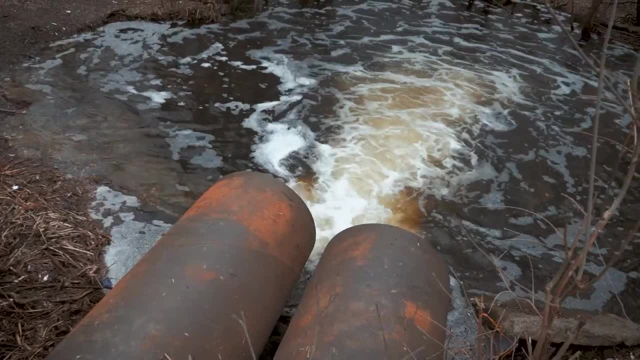 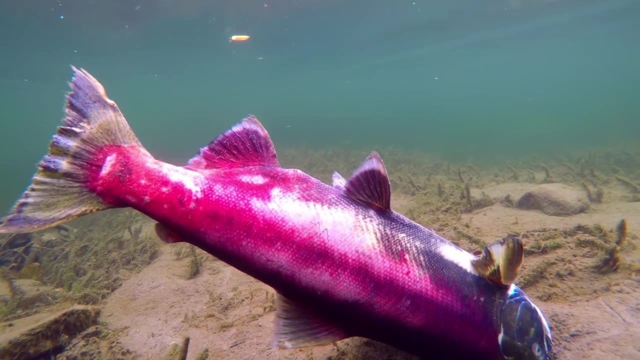 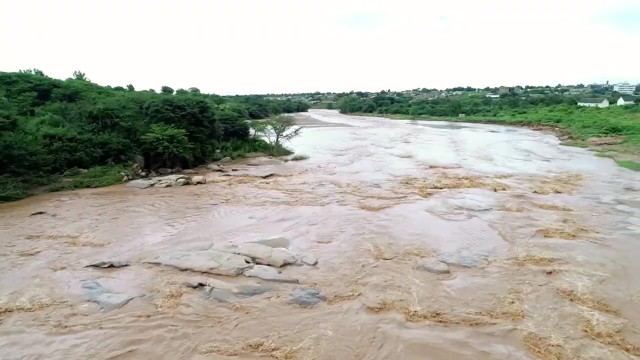 It will also seep into the soil and contaminate the surface water, resulting in a detrimental impact on aquatic life. This will cause pollution in the surrounding streams, rivers and lakes. Furthermore, it may also cause problems for those who rely on wells or groundwater to survive. 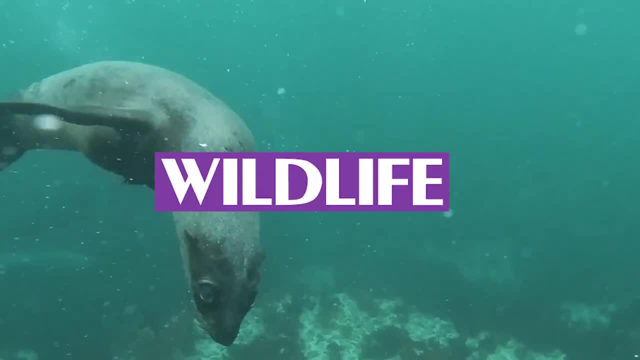 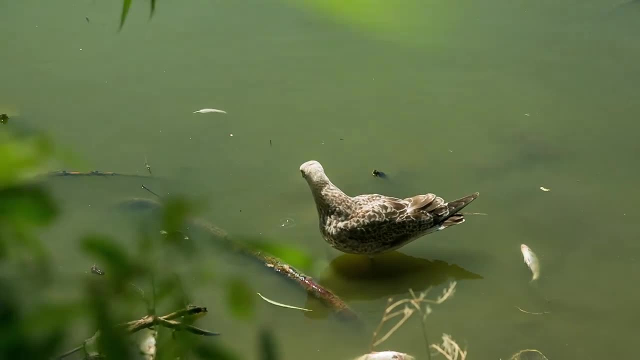 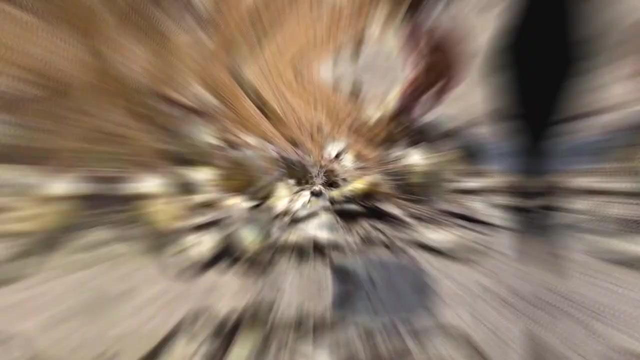 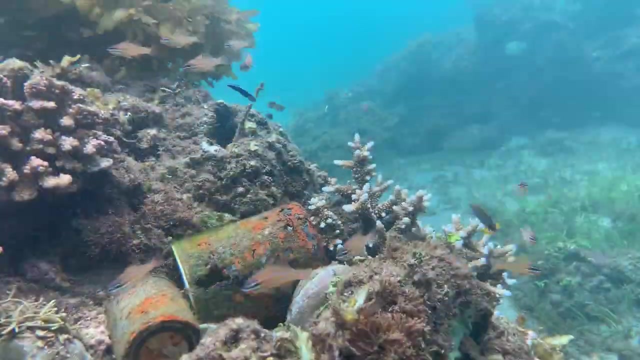 Wildlife Ecosystems differ from place to place. However, one of the most dramatic repercussions of our worldwide trash crisis is in our marine life and rivers. Simply put, it has an impact on people who rely on the ocean for a living. Ocean organisms are unable to distinguish between what is and is not food. 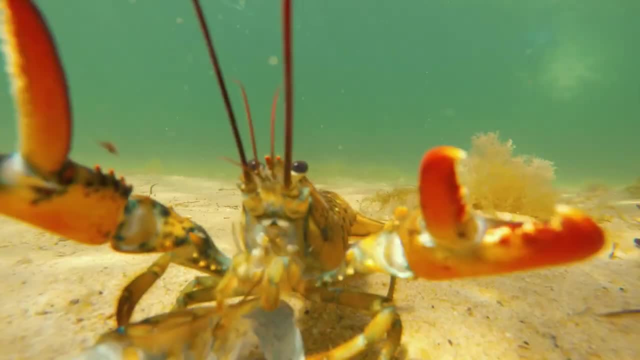 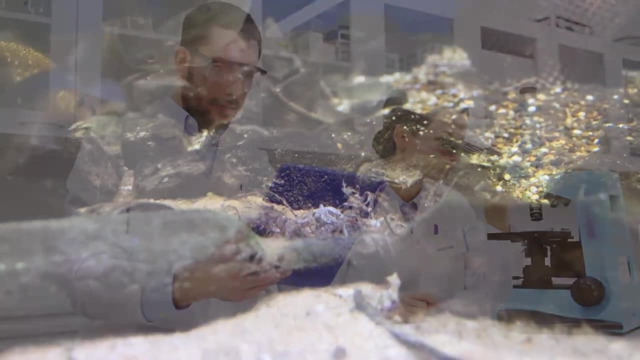 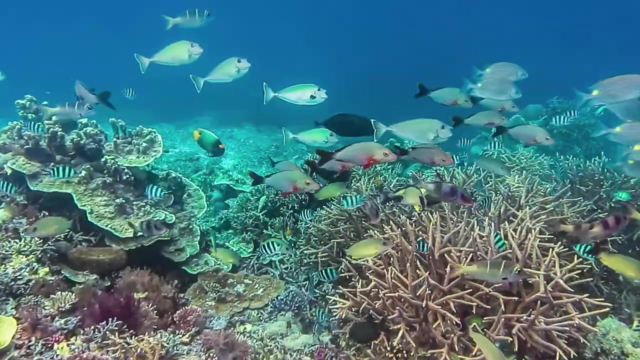 They devour waste, which kills them because the aquatic animals cannot metabolize it. This has an impact on many aquatic animals and organisms. Scientists have discovered numerous plastic particles in over a thousand different species. Many marine species do not have high acidity levels in their stomachs to break down the material consumed. 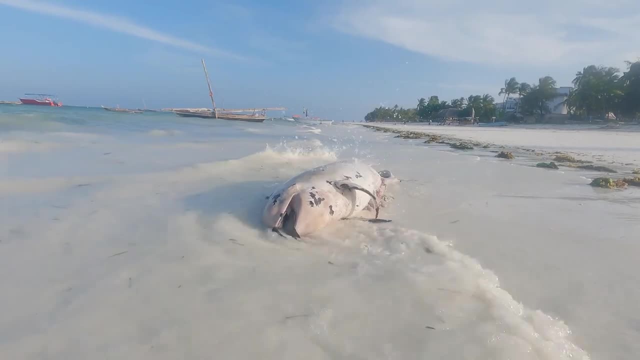 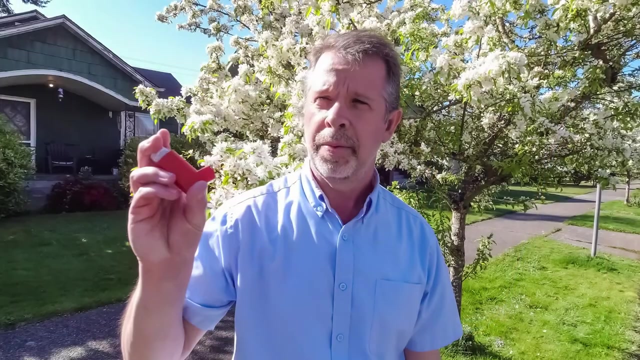 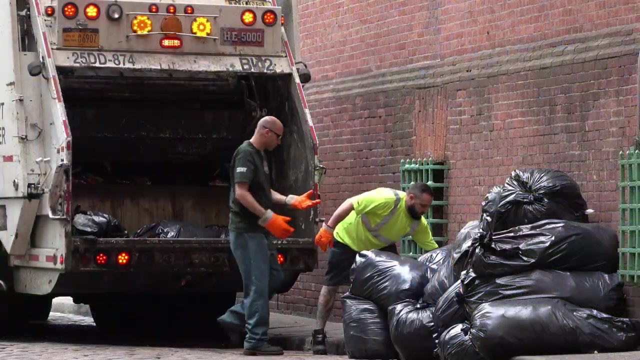 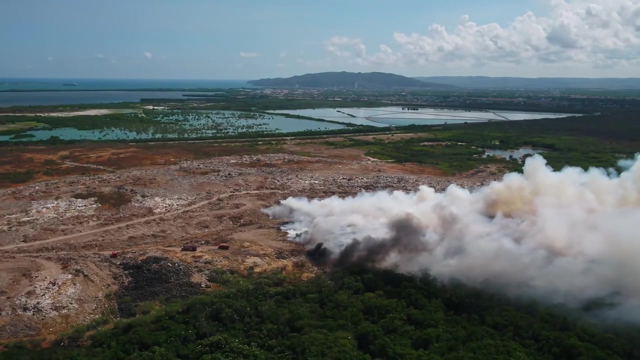 resulting in starvation after the ingestion of rubbish or plastics. Because of our inactivity, human health is affected. We continue to generate vast amounts of waste And we fail to dispose of it. The more rubbish we generate, the more the emissions are released into the environment. 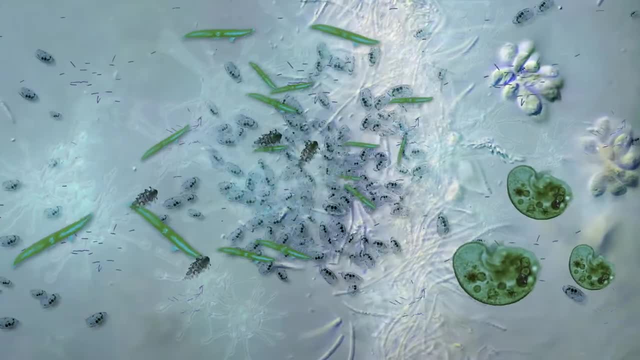 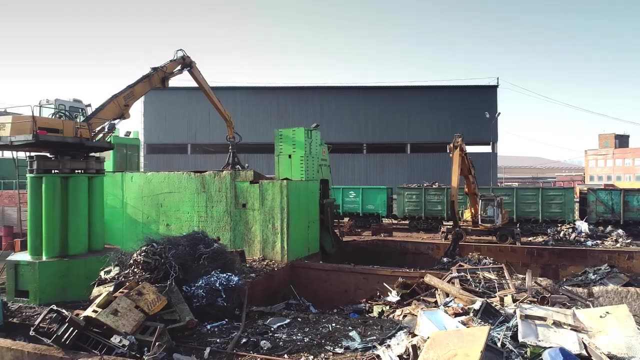 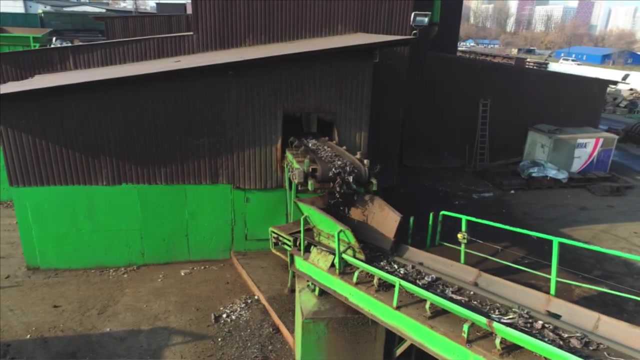 Trash waste is an ideal breeding ground for bacteria, insects and vermin. We must remember that just because we toss something away does not imply it is no longer there. It usually ends up somewhere that is harmful to the environment. Recycling can assist to mitigate this. 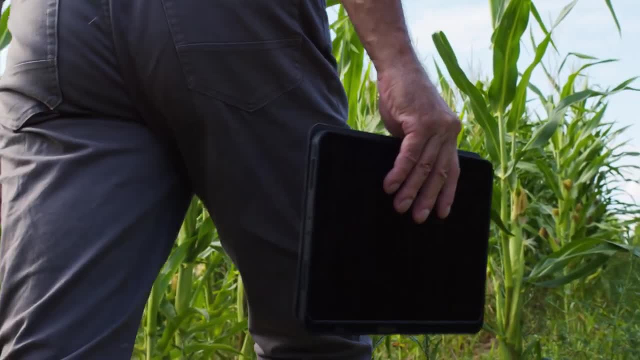 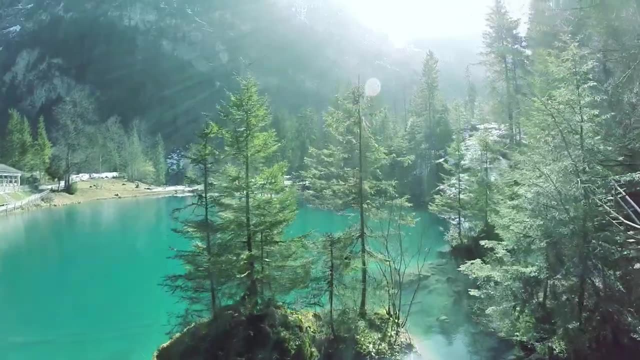 We must avoid these negative effects and safeguard the ecosystem from contamination and pollution. If you like this video and would like to hear more, be sure to press the subscribe button.